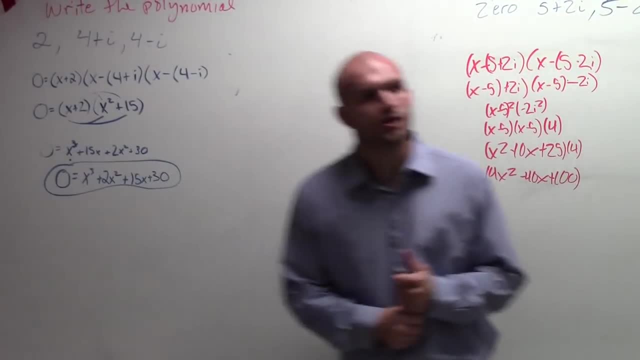 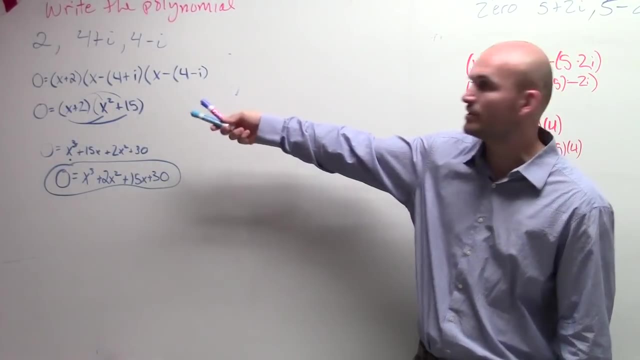 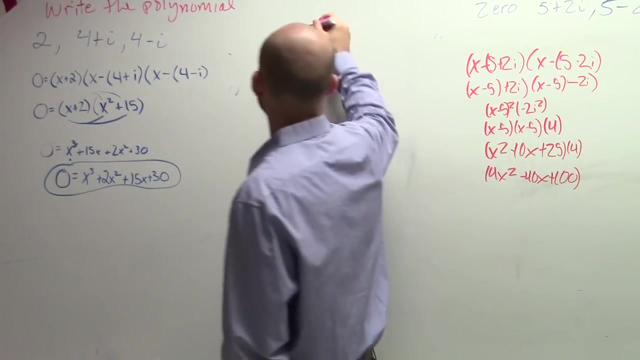 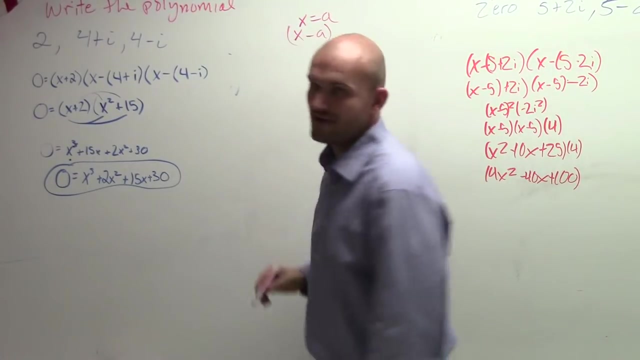 How I want you guys to do this. So I said: write the polynomial. alright, Now you're giving your zeros. Remember, ladies and gentlemen? we talked about this. The student did a great job. We go from zeros to factors. That's the hardest part, right there. Alright, You gotta write from zeros to factors, because, remember, if I have x equals a is a zero, then x minus a is my factor. So the student did a great job. They wrote down the correct factors. 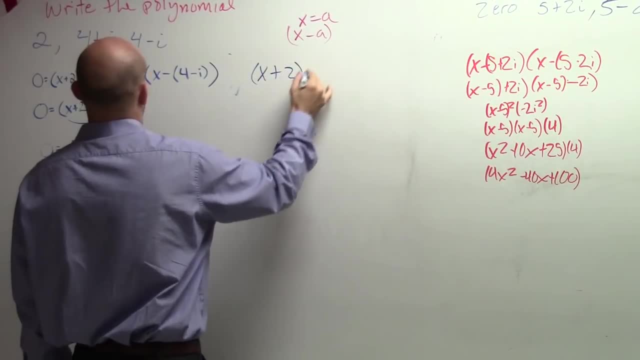 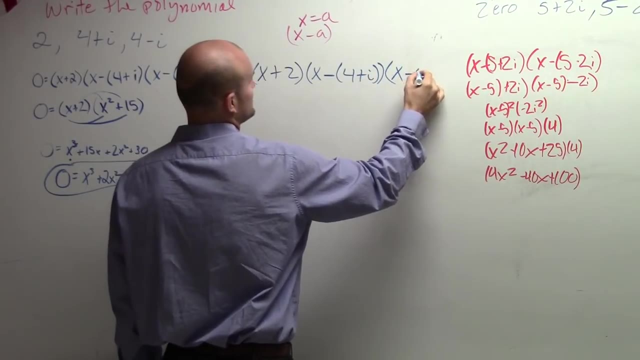 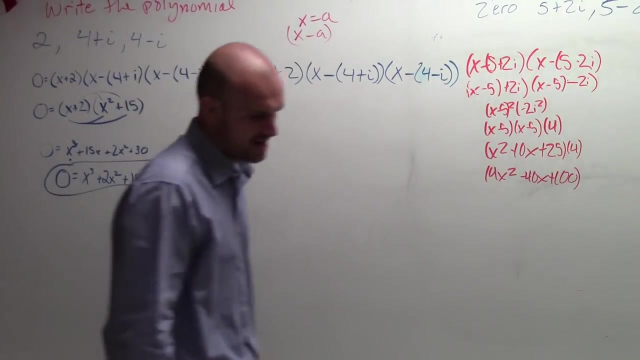 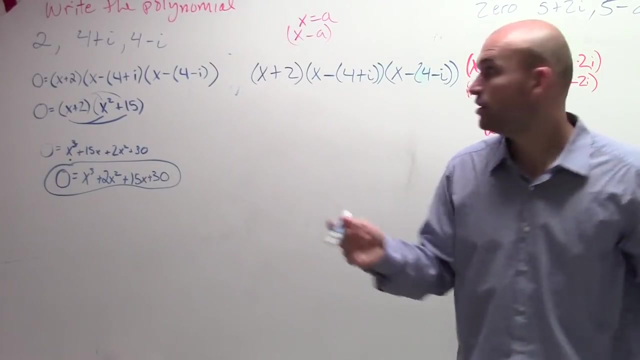 I'm just going to write them again, just because I'm going to do my math over here. Make sure you kind of have the correct parentheses so you just don't get confused. Okay, so that's what the student has, But remember that was the factor form. Now remember the factors multiply to give you your polynomial. So we're actually not going to set this equal to zero, We're actually going to set this equal to one. 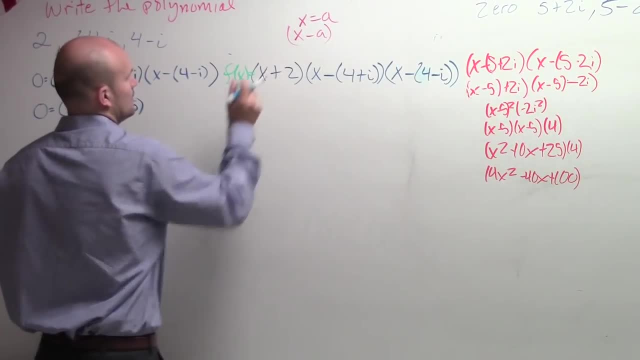 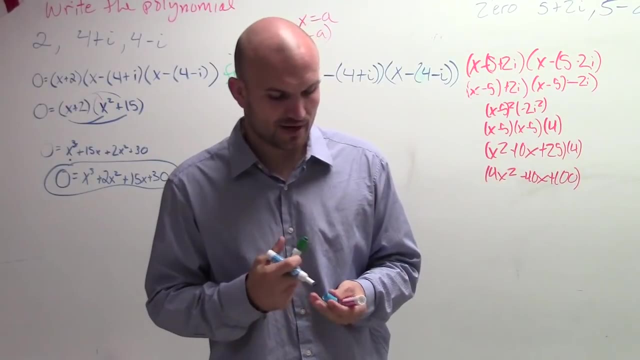 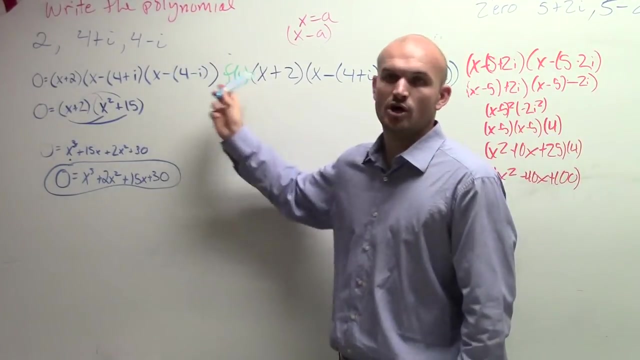 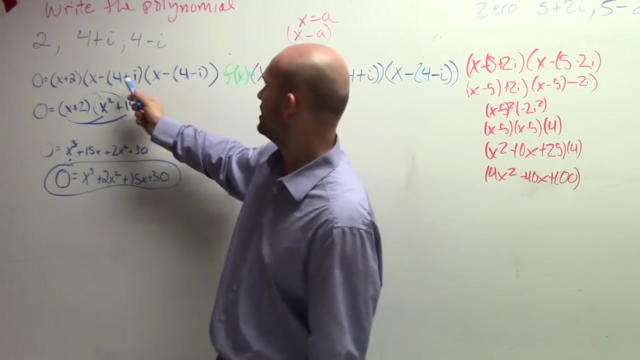 So we're actually going to set this equal to f of x. Okay, So the student did good from there. Now what we need to do is the hard part. Maybe we need to multiply this, And this is where we made the mistake. Alright, And it's very difficult. if you don't do this trick, Ladies and gentlemen, you can multiply this out, But remember: this is four plus i times a negative. four plus i. That's actually. that should be x minus. Yeah, that's right. This is four plus i times four minus i. 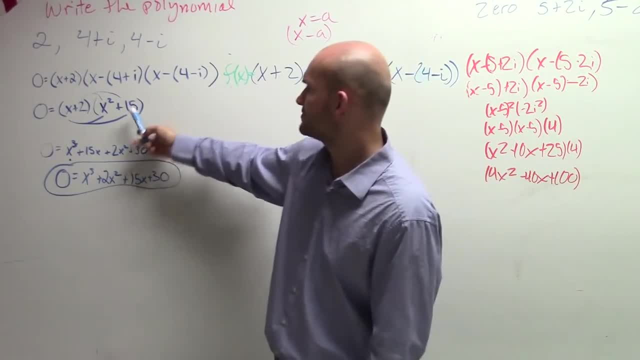 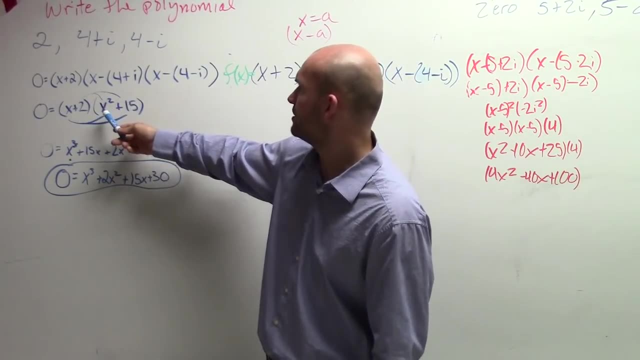 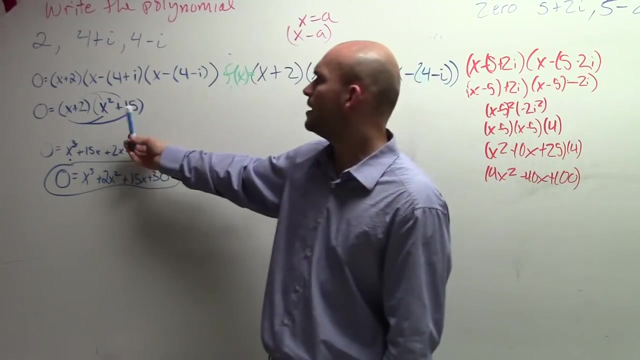 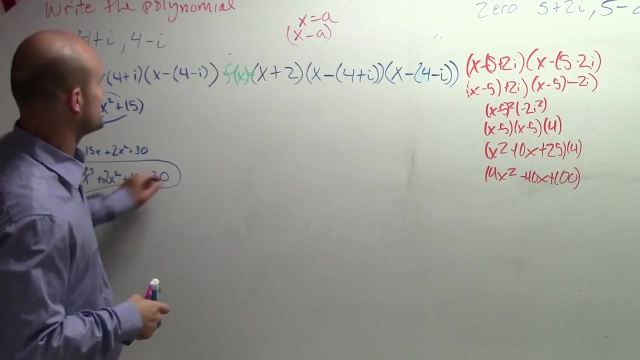 Alright, Actually we're going to get x plus 15.. We're getting very close, But we made a mistake. x squared, Shouldn't the x? shouldn't it be x minus two? Because I have x? Let me just go through it. Let me actually see, because they're close but they're not right. I don't know where they made the mistake. Let me look at it. 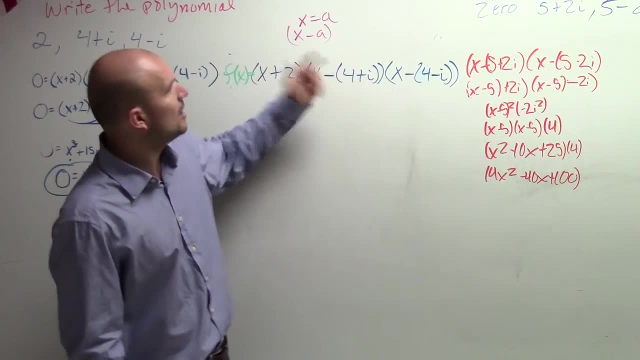 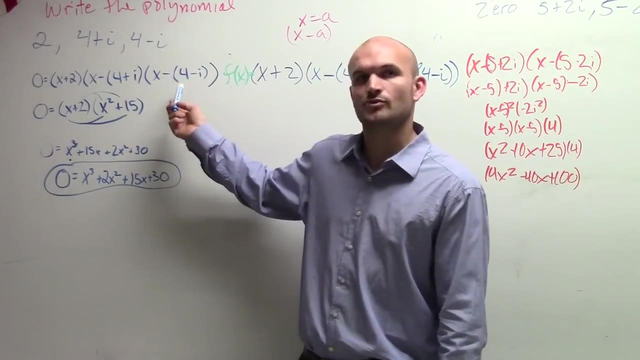 What I would like to do rather than multiplying. Oh, here's what they have, Here's what they did. They did a difference of two squares, but they didn't multiply everything out. These are not a difference of two squares, right? So they multiplied these two terms correctly and they multiplied these two terms correctly. 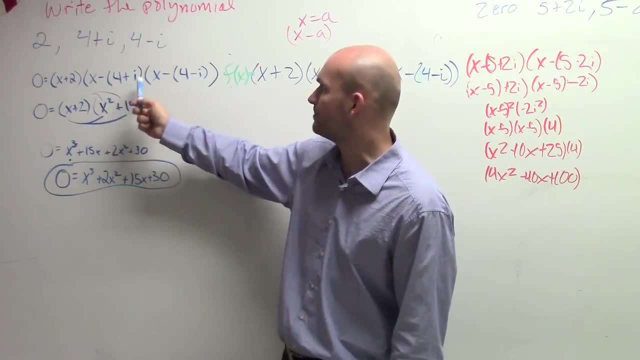 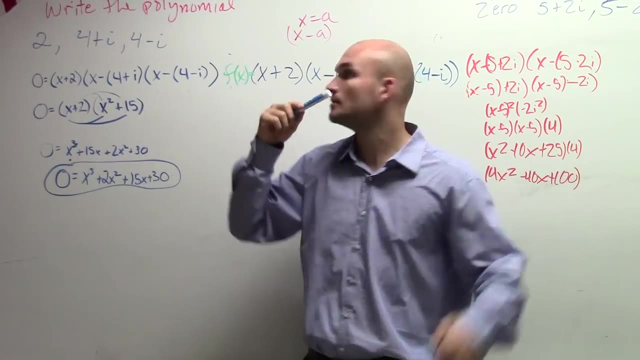 But they didn't multiply x times four minus i. Nor did they multiply x times negative four minus i. Right, You've got to use FOIL x minus two. Huh, Firstly, x minus two, not x plus two. That's what I just said. 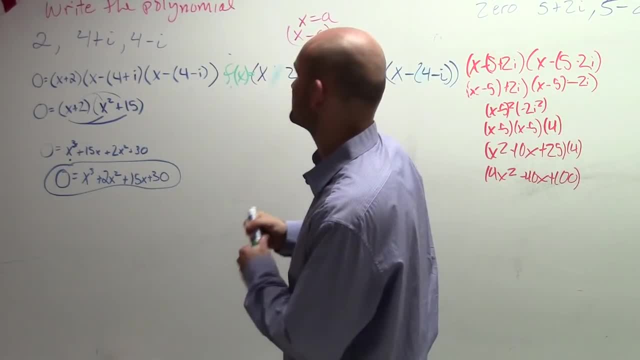 Oh I, I just said that, Oh from here, Yes. Yes, x minus two, Thank you. I was actually just saying: Oh I, I just said that, Oh, from here, Yes. I was actually just kind of looking at it. 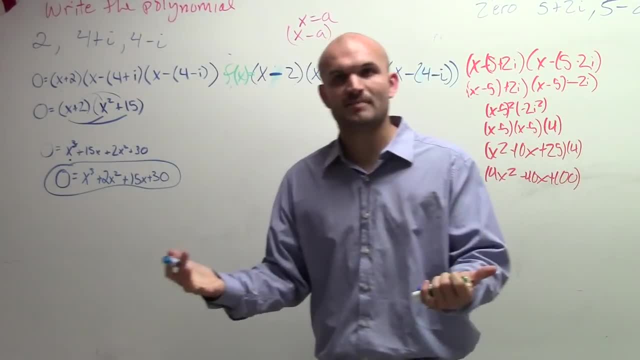 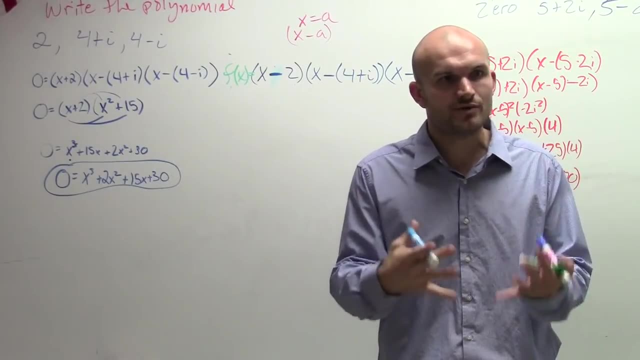 Yes, Since the zero is positive, it would be x minus two. Thank you, But where the student made the mistake is, they only multiplied the first two terms and the last two terms. Ladies and gentlemen, you can only do that when you have a difference of two squares. 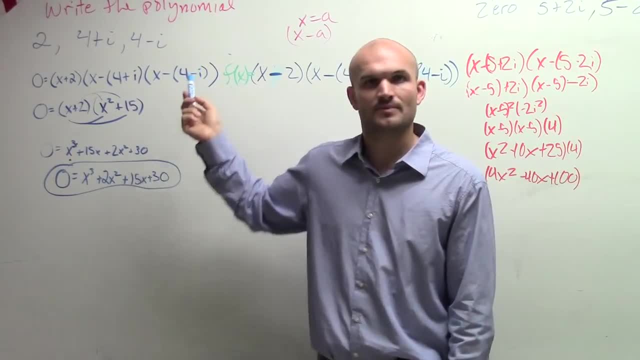 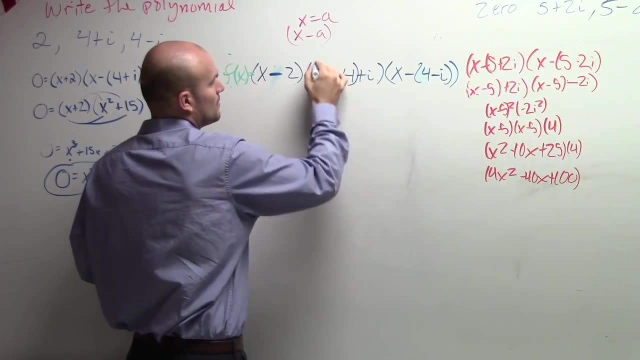 This times. this is not a difference of two squares. What is a difference of two squares? Well, what we can do is I'm going to rewrite my parentheses If I put my parentheses for the first two terms rather than for the last two terms. 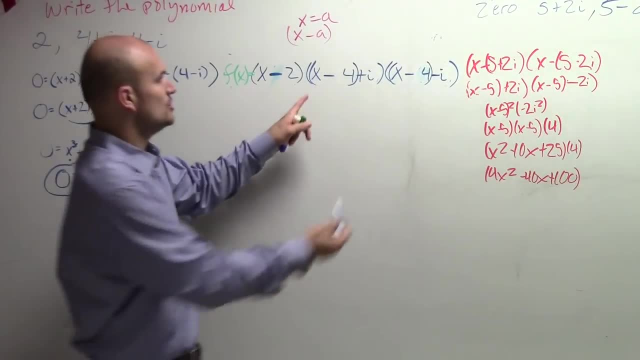 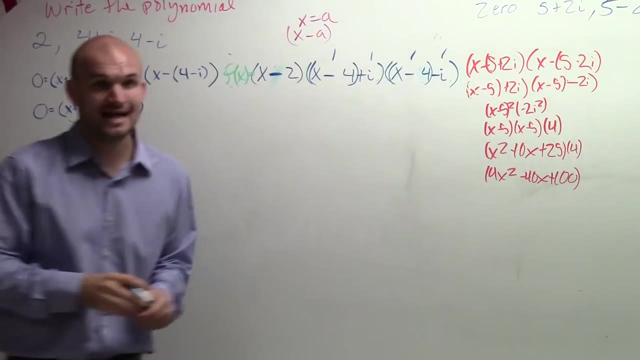 I now create a difference of two squares. Notice my first two terms. are those the same? Yes, Are my last two terms the same? I and I? Yes, Do they have a difference of signs between them? Yes, Now I can use difference of two squares. 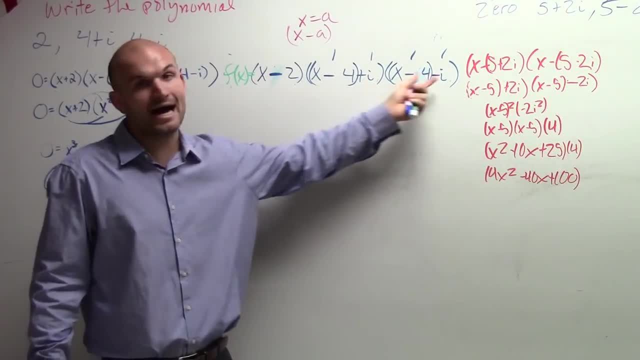 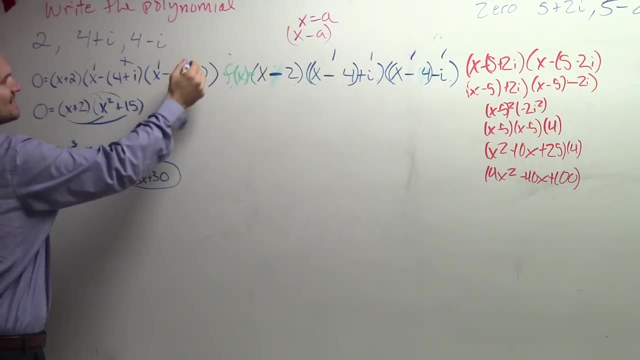 where I only multiply x minus four times x minus four and I times negative, i Over here. these are the same, These are the same, These are not the same Right. So To multiply these you'd have to do FOIL. 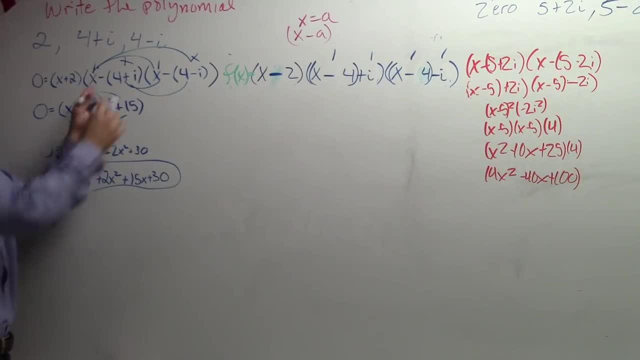 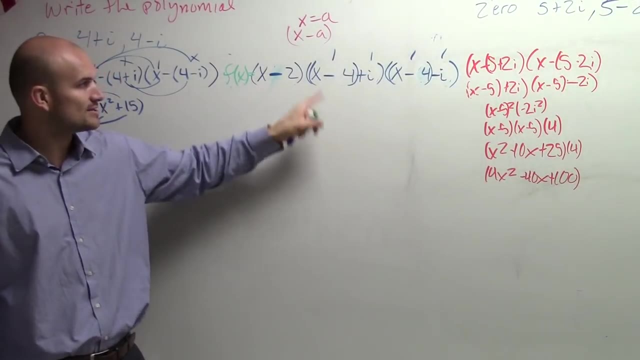 Multiply every term, times every term, You would still get the same answer, but you've got to make sure you multiply everything by everything. OK, So what you did, the shortcut was without having a difference of two squares. So I rewrite my parentheses. 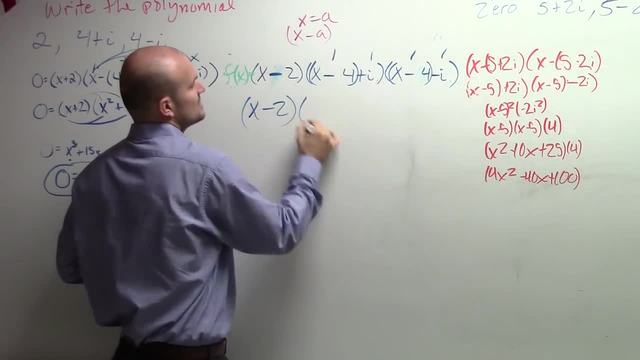 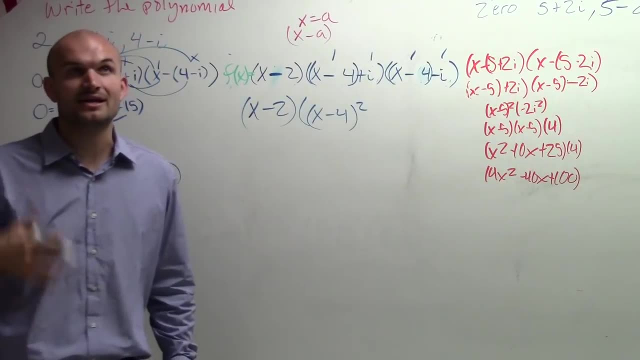 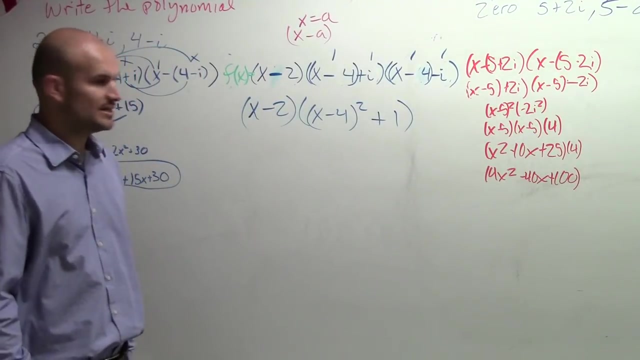 Now I have difference of two squares, So I have x minus two times x minus four squared. plus i times negative. i is negative, i squared, i squared is negative one, so it's going to be plus one, Right? Does everybody see this? 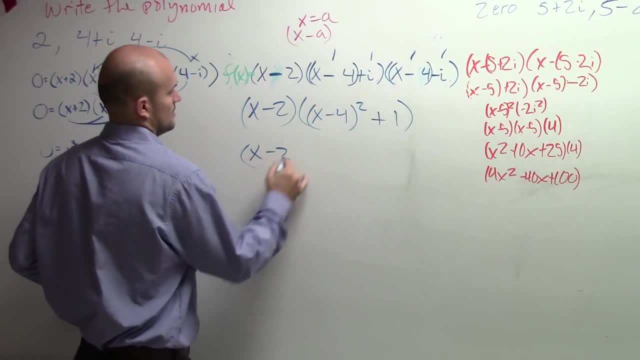 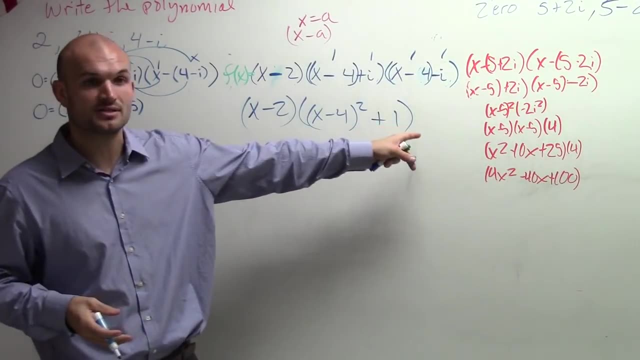 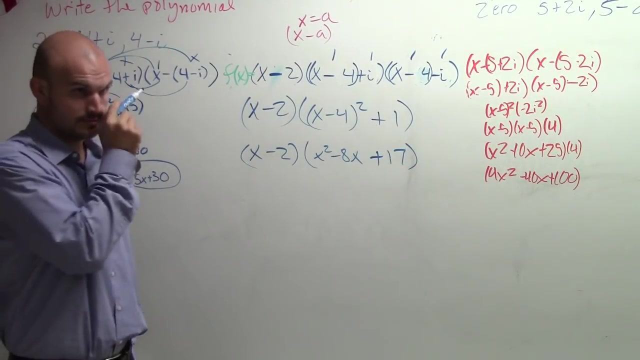 Now what is x minus four squared? It's going to be x squared minus 8x plus 16.. Right, But now I have the i plus 1, so it's going to be plus 17.. I thought that was on the outside of the parentheses. 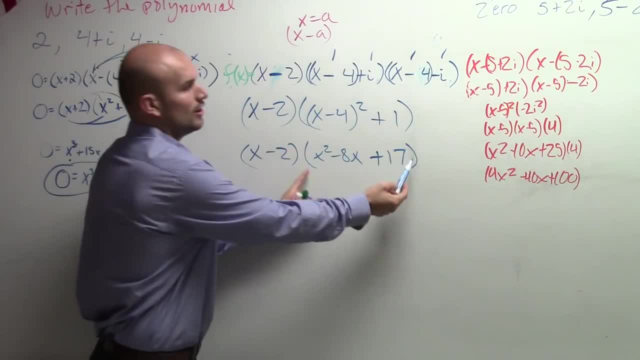 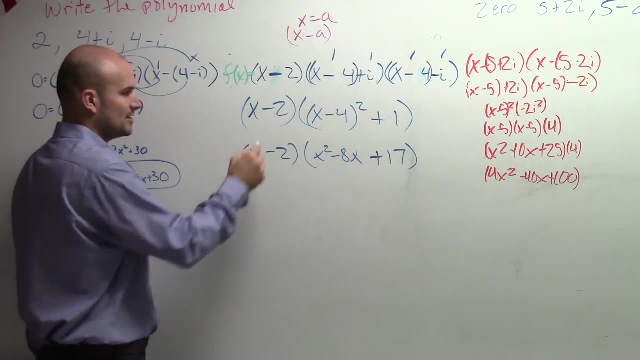 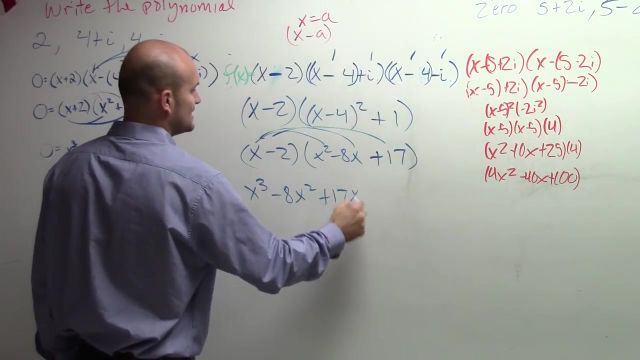 It's inside of these parentheses, Right? So now all of this is multiplied by this. So again I have to use distributive property or multiply a trinomial times a binomial, So x times x times x. So I get x cubed minus 8x squared plus 17x. 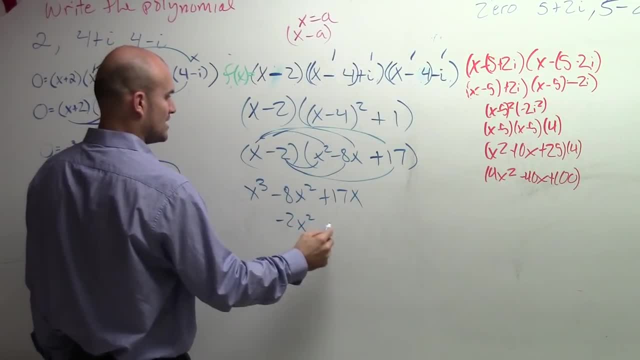 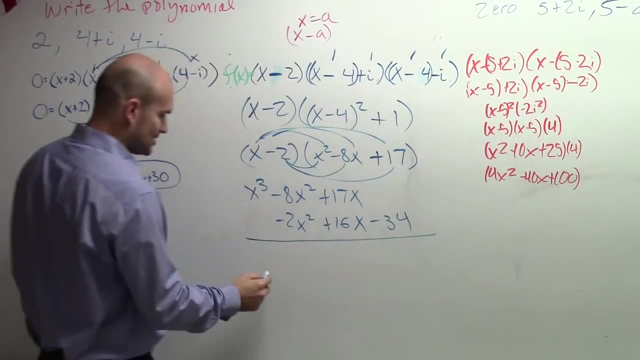 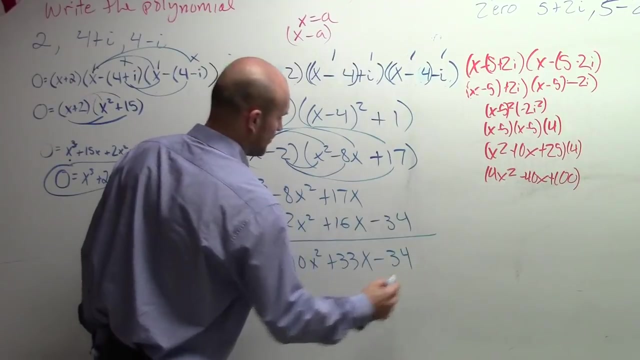 Multiply it times every term Negative: 2x squared plus 16x minus 34.. Combine my like terms: x cubed minus 10x squared plus 33x minus 34. 33. There we go, Good, Everybody see it. 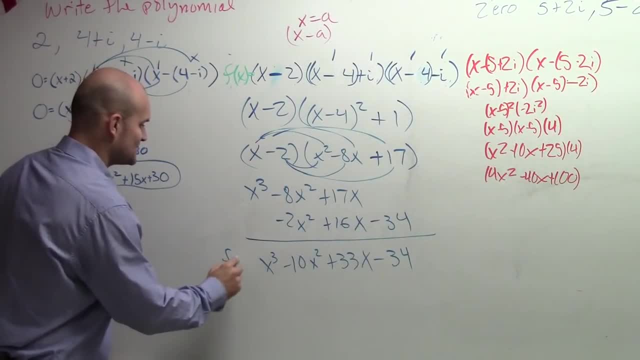 So then, that's what f of x equals. See it Make sense? Yes Questions, Go for it. I did this. I multiplied this out: x squared minus 8x plus 16, because negative 4.. Remember, this is x minus 4 times x minus 4.. 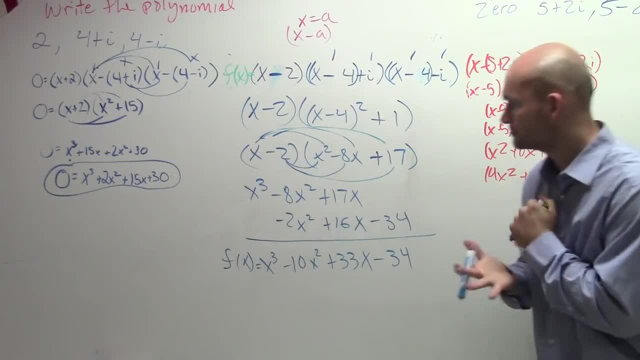 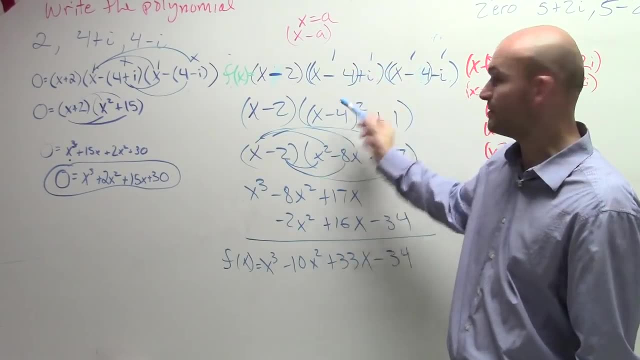 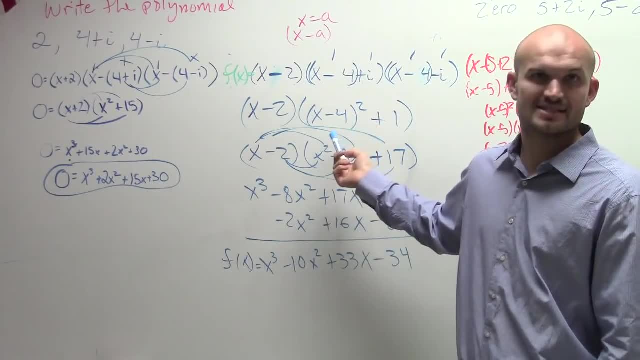 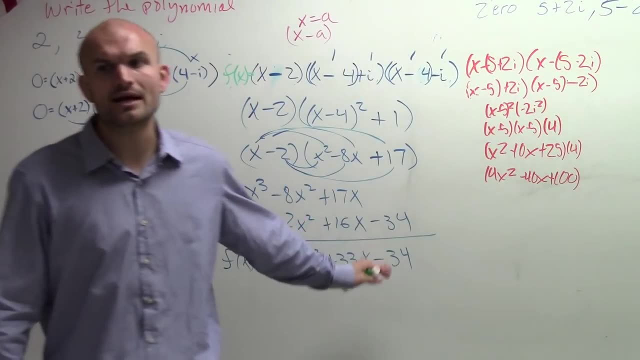 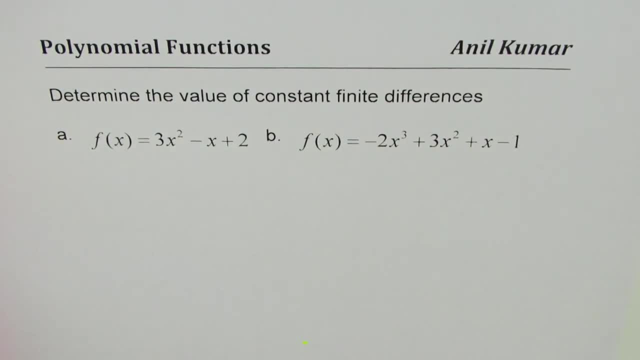 Amanul Kumar in this video will learn a formula to find constant finite difference from the given equation of a polynomial. The question here is: determine the value of constant finite differences. We are given two polynomials. A is f of x equals to 3x square minus x plus 2.. B is f of x equals.